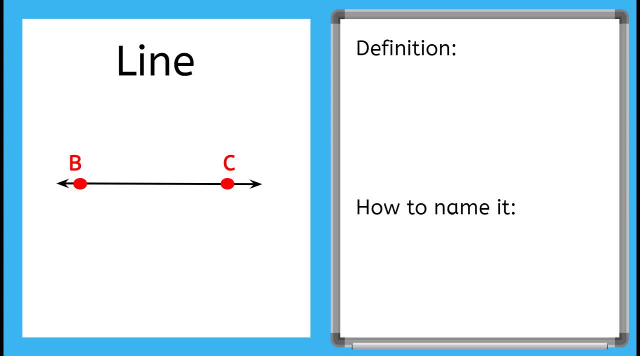 Now, this is a line. While this line looks like a straight line, it's really made up of an infinite number of points, or a lot of points, a whole collection, that go on indefinitely or forever, in both directions. We know this because of the arrows on either end. Notice that two of the points on the left side of the point are in their label. Notice that two of the points on the right side of the point are in their label. Notice that two of the points on the left side of the point are in their label. 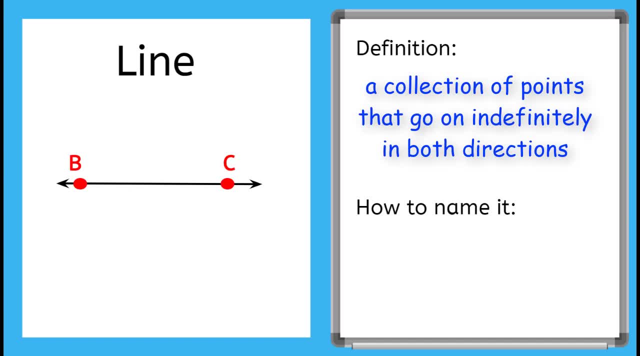 Notice that two of the points on the left side of the point are in their label. Notice the arrows on each of the points on the line have been named: point B and point C. To name the line, we will use the letters for the points with a symbol above them and the symbol is a line. 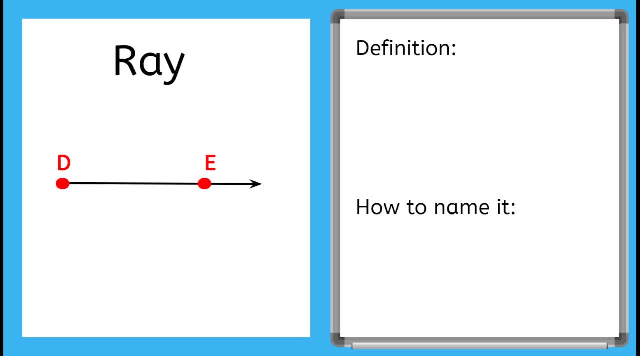 Now we have a ray, like a ray of sunshine, that starts at the sun and spreads out forever. a ray has one end point but extends in the other direction infinitely. Notice that there are two points on this ray. One of the points is at the end, point point D, and point E is on the ray. 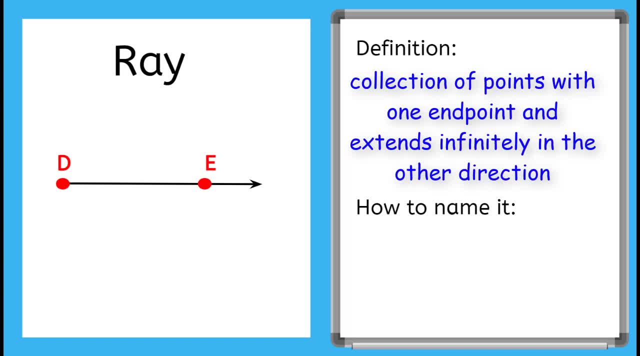 To name the ray we use the two points and a symbol. The symbol looks like a little ray above the letters. Our next geometric shape is a line segment. We know that this is a line segment and not a line because it has two end points. 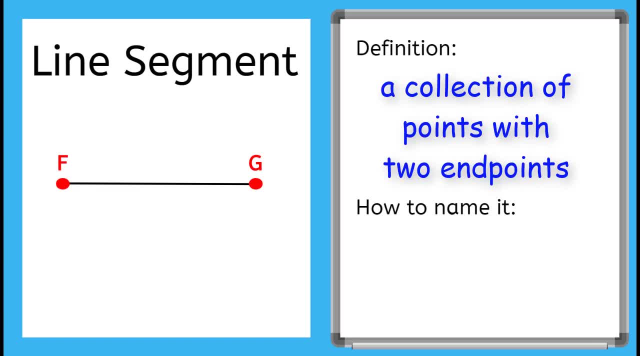 We see the two points here and the end points have been named: point F and point G. We can name a line segment by using the name of the end points with a symbol on top. The symbol is a small line segment. Intersecting lines are two lines that cross each other at a point. 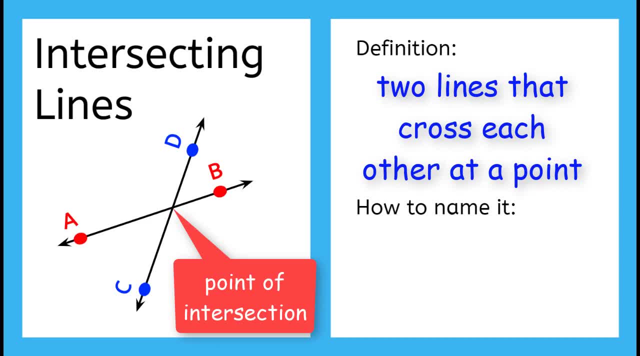 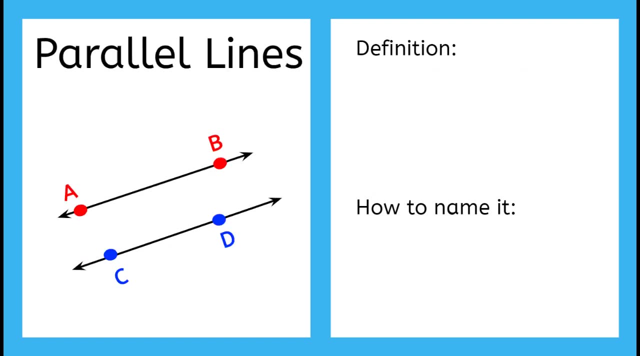 The point where they cross is called the point of intersection. We would name this intersection with the names of both lines. So line AB is intersecting line CD. Parallel lines are two lines that will never, ever cross each other. They are equidistance apart.